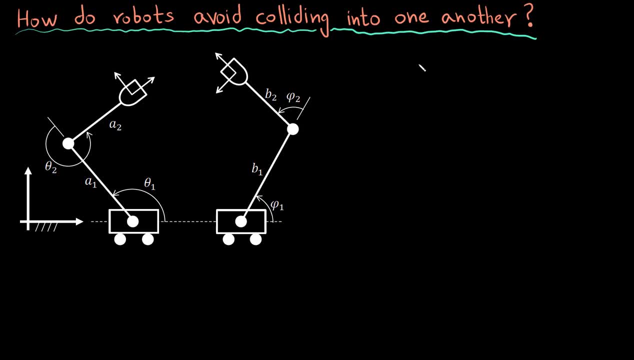 express one moving frame with respect to another. So how can I express one moving frame- let's say my moving frame M1- with respect to another moving frame? In order to explain why that is, I have chosen this example. In this there are two robots, mobile robots. they are moving about and there is a fixed frame placed here. 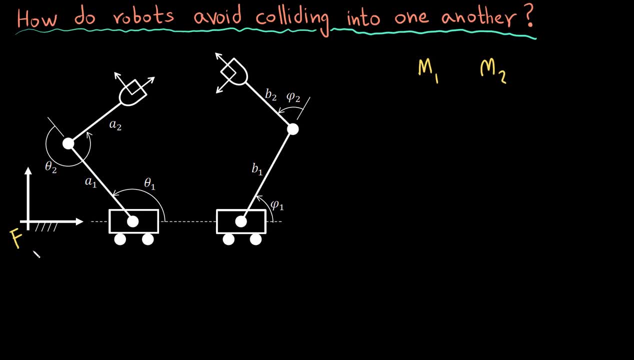 So if I know distance, how far the first robot is from the fixed frame and if I know how far the second robot is from the fixed frame, then I can simply find out the position and orientation of this moving frame. let me call this m1 with respect to the fixed frame. So I can find out this. let's say i call this h of A. 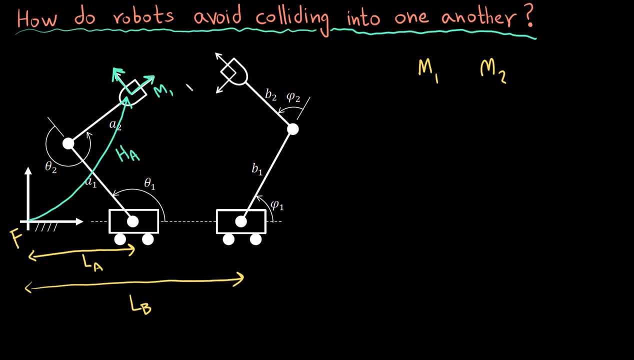 homogeneous transform which takes the fixed frame to the moving frame one, and then, if i can find out the position and orientation of this frame, let me call this m2.. So, if I can find out the homogeneous transform this moving frame will be: takes the fixed frame to the M2 frame, I call this HB and finally I take another. 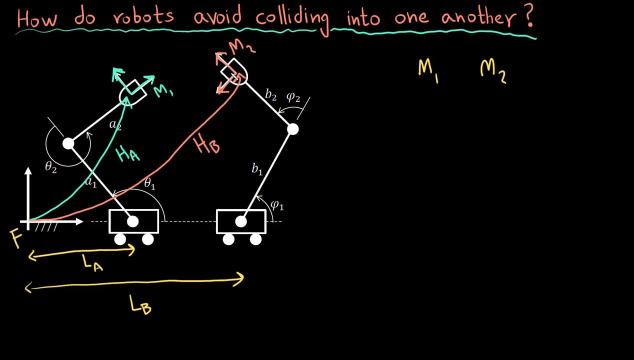 homogeneous transform that takes the M2 frame and puts it to the M1 frame, and let me call this HBA. so homogeneous transform that takes the B frame or the M2 frame to the A frame. what I mean is, if I go about in circle, I can say that 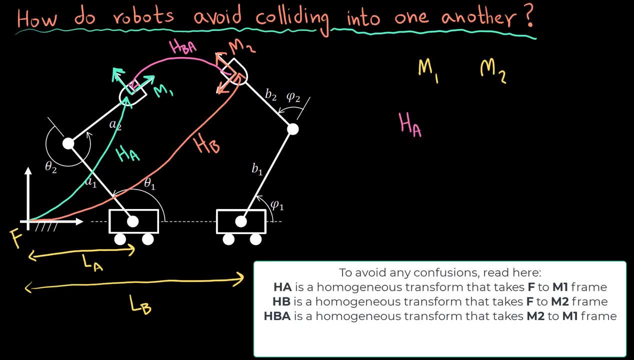 HA. so the fixed frame to the HA frame here would be equal to HB frame times the HBA frame. so what this means is that HA takes the fixed frame to the M1 frame and HB takes the fixed frame to the M2 frame and HBA takes it. 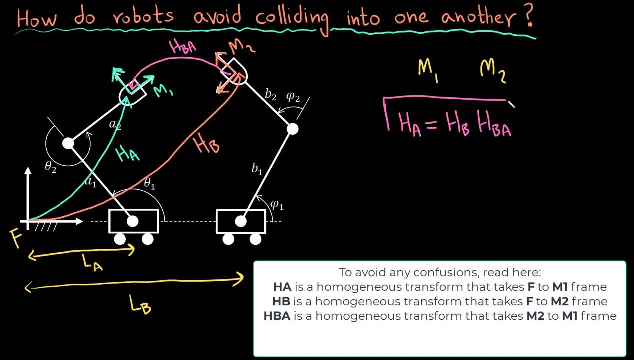 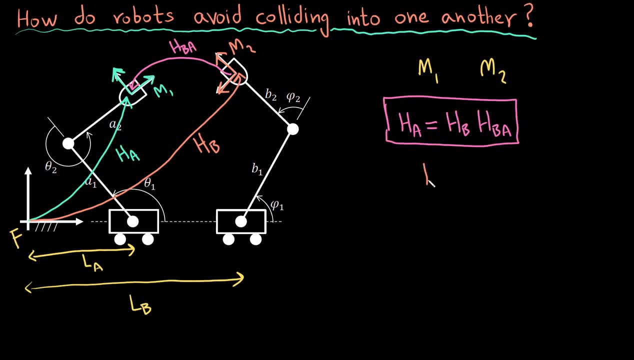 back to the M1 frame. so this right here, the terms on the left and the right are equal. and now from this, if I make HBA the subject, so I would get HB, inverse times, HA, and this HBA, the homogeneous transform represented by this, would be: 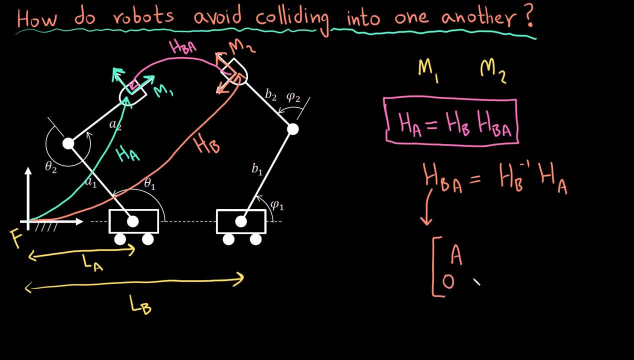 of the form of a rotation matrix, here two zeros and two terms. here let me call it this DX and DY and a 1. if I am able to get this from this homogeneous transform, I can figure out DX and DUI right, and what this would mean is this: DX would simply be how far? 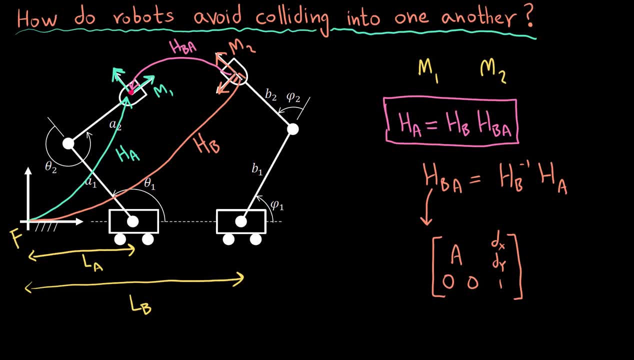 this. this origin is from this point in X. so this would be my DX and this will be my DUI. so this right here would be my DX and this right here we'll do you my dy. and, of course, when this dx and dy would be 0 and 0, then the two end factors would be: 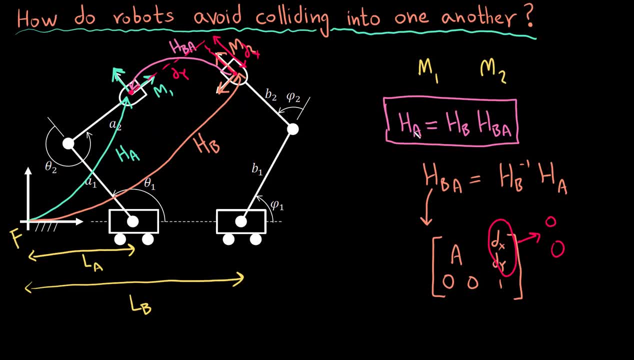 colliding and on top of each other. so all i need to do is i need to find out hba, a homogeneous transform that takes the, the m2 moving frame, to the m1 moving frame. now, before we move on to the formal question for this, let me bring something to your notice. so we know that the a matrix which 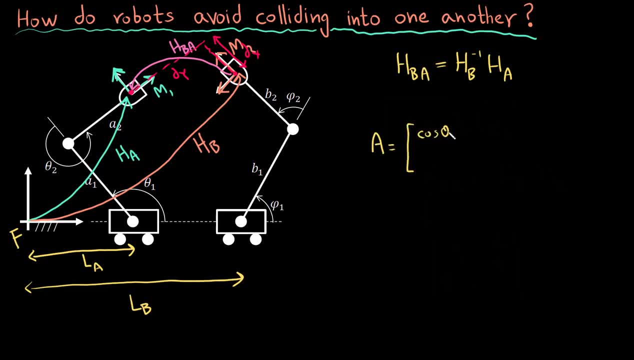 is the rotation matrix is always of the form of cosine of theta, sine of theta, minus sine of theta, and cosine of theta and the a inverse of this matrix is just the a transpose of this matrix. so a inverse would be equal to the a transpose which would come out to be cosine of theta. 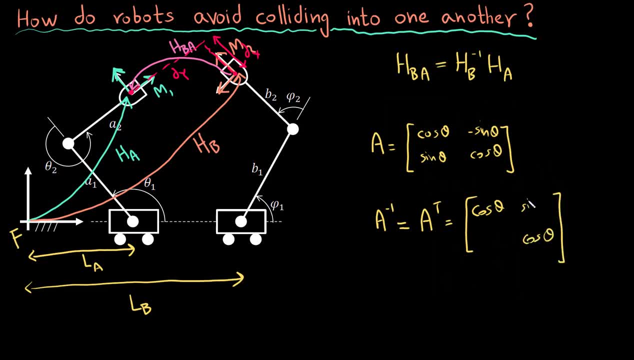 cosine of theta here, and this is going to be sine of theta and minus sine of theta. if you want to verify, you can do this, since you know that a matrix times its inverse is always equal to the identity matrix. so you can solve this out and prove that this, indeed, is true. 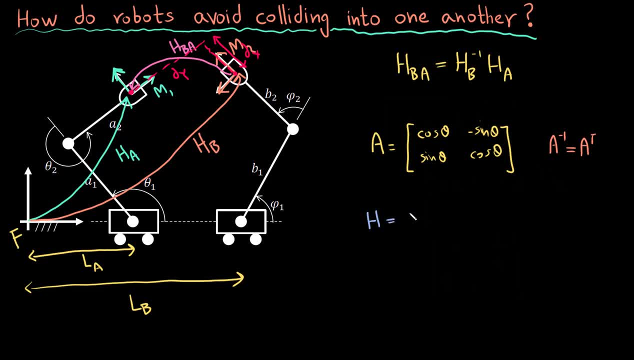 now, what about the homogeneous transform? so we know that the homogeneous transform is of the form of sine of theta and sine of theta. this is going to be sine of theta and minus sine. that there is a rotation matrix here, two zeros. there is a displacement term here and one. 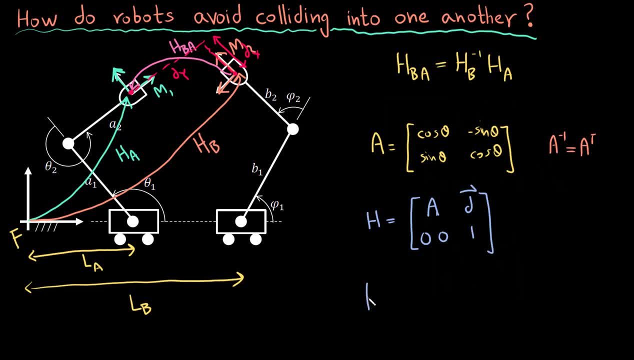 and if i find out the inverse of the homogeneous transform, i figure it out that it is of this form: a transpose zero, zero minus a transpose times d and one. and of course you can verify this by using this equation: h times h inverse should give you the 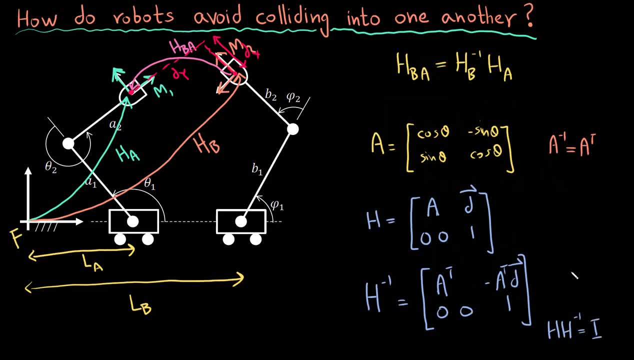 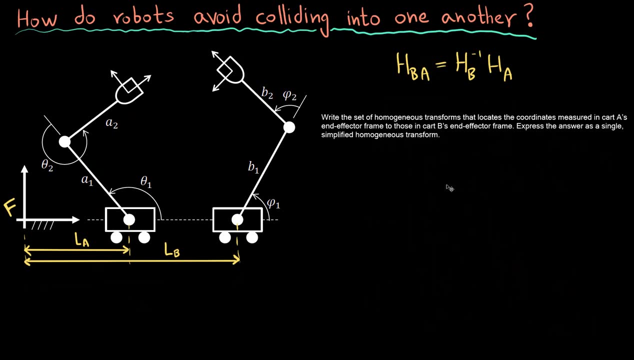 identity matrix. you do not actually need to know this and this, but it's always good to know this just in case if you get stuck somewhere. so this might help you out. so this right here is the question that i have, and it says that i need to explain the equation of the homogeneous transform. 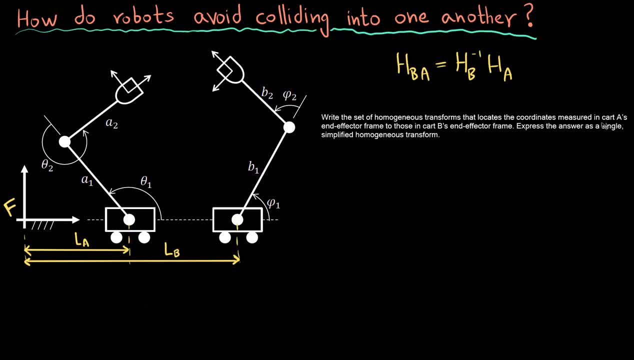 and it says: express the coordinate in cart a's and a factor frame to those in cart b's and a factor frame. all this means is that i need to find a homogeneous transform that takes this to this, which is the h? va that we wrote here and it also asks us to express. the answer is a single, simplified, homogeneous transform. 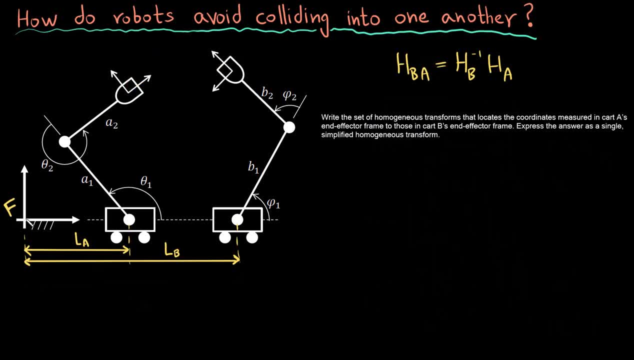 so i know that my first homogeneous transform that i need to find out this HA. so my HA is going to be the multiplication of this homogeneous transform, h1, which takes the fixed frame to this, then the one that takes this to this h2 and the one that takes this to this h3, so HA would just be equal to. 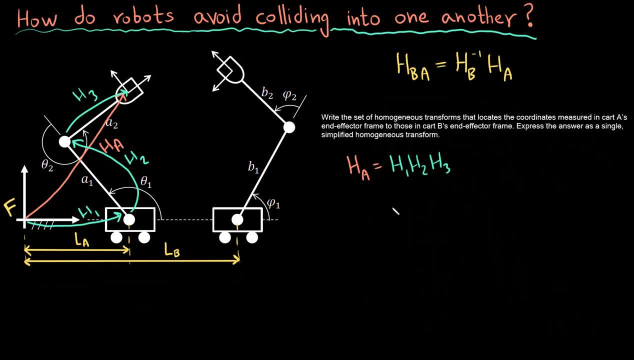 h1 times h2 times h3. and if I write it in a more expanded form, I can see that this is going to be a of theta 1- 0 vector transposed and it is going to be a 0- 1. my h2 is going to be a of theta 2, 0 and 0 and a 1- 0- 1. 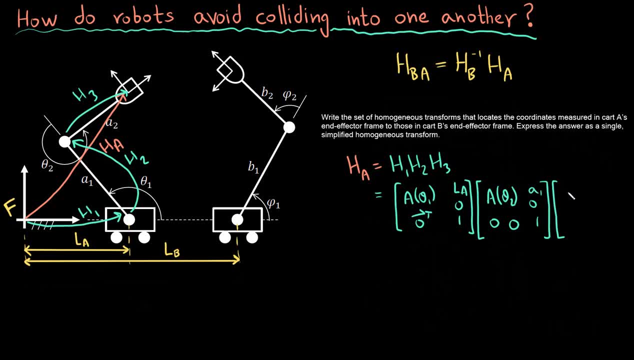 and and my h3 is going to be now we, you can see that your frame is right here and taking it from here to here. there is no rotation involved, so it is just going to be an identity matrix. so 1, 0, 0, 1, 2 zeros and this is going to be a 2, 0 and 1. now 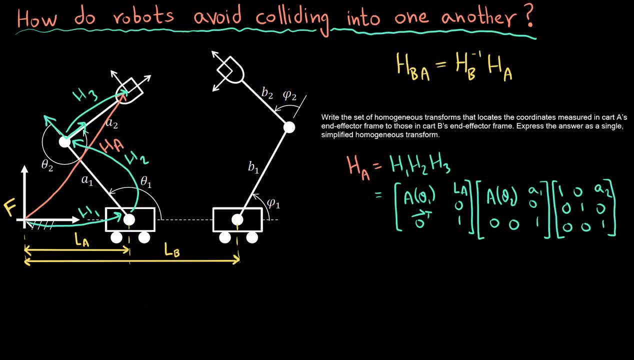 for the, for this one, which is, which takes a fixed frame to this frame right here, the HB, I can say that H B would be equal to the met, the homogeneous transform. that takes this to this first. so let me call this H 4, then this to this H 5, and 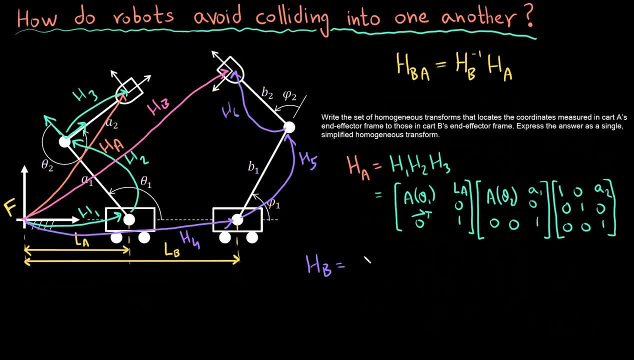 then this to this H 6, so as we would be equal to H 4 times H, 5 times h6, which is just going to be equal to a of 5 1 0 0, a B 0, 1, a of 5 2 0 0, then 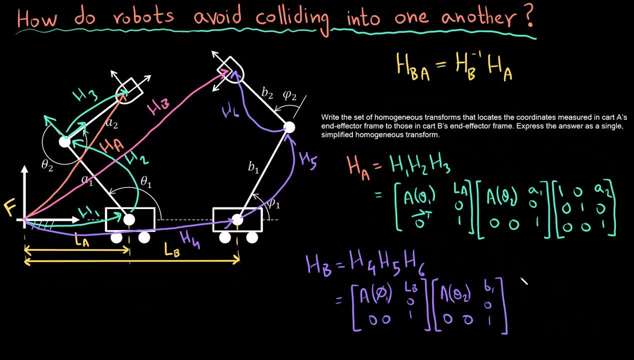 this is going to be B 1 0, 1 and again there is no rotation involved. so it is going to be 0 and identity matrix here and 0 and P 2 0- 1. now I have H a, I have HP, so I know that H a is equal to H B times H B a, where H B is the matrix that. 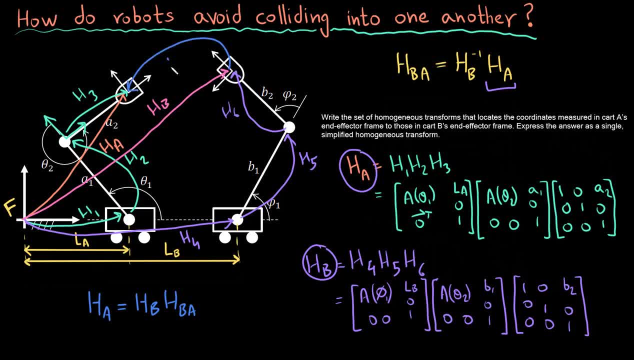 homogeneous transform. sorry, that takes H B to this H B, and this is what we need to find. so if I make H B the subject, it is this: H B- inverse times H a. and now I can obviously do this using pen and paper or, in this case, my drawing tablet, but a. 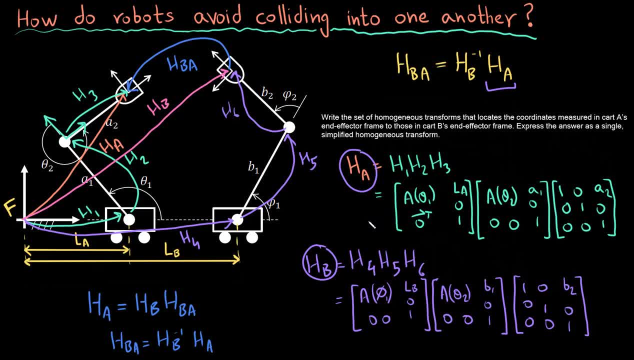 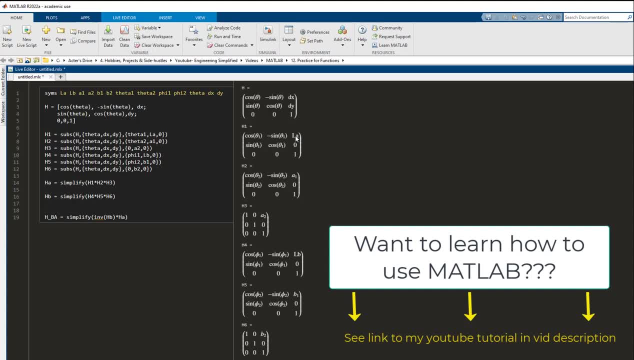 better approach would be to use a software for this. so let me pull up my MacDab really quick. if you don't know how to use MacDab, I have a complete tutorial on MacDab. I am going to put a link down in the description if you want. 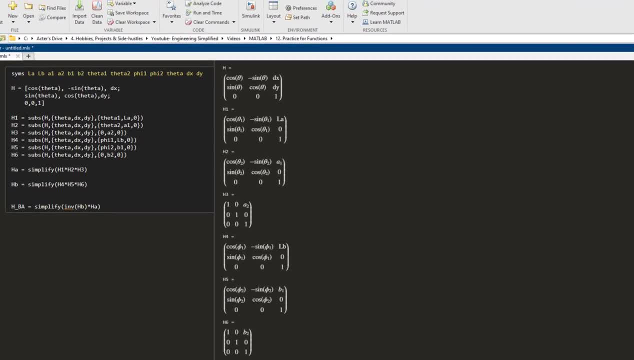 to go down there to it. so I have just input all these H 1, X 2, X 3, 4, X, 5 and 6, and you can see the output on the right at 5 and X 6, and I have calculated H a, H B and then I have